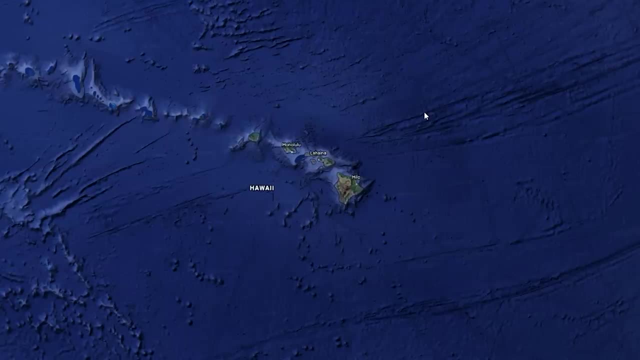 Alaska, Yeah. so I don't think anyone's taking over Alaska. And then Hawaii. Come on, They're not gonna, You're, you're no. No one's gonna come out here. It's too far and they're, they're chill. 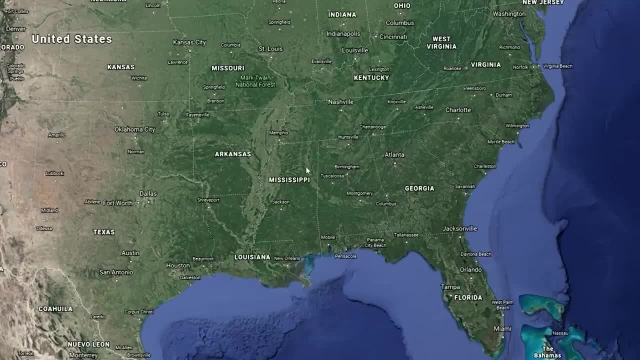 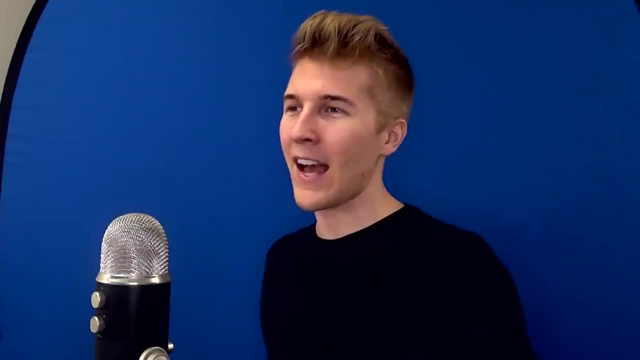 Like overall regions. Obviously, I would assume deep south gonna do real good here, But at the same time a lot of them would do so good. They'd probably take each other out and that'd be kind of an issue. And yeah, I'm sorry in advance, but these flat states in the middle, I just there's. 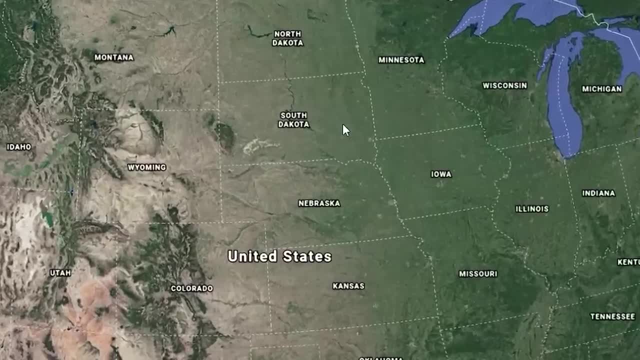 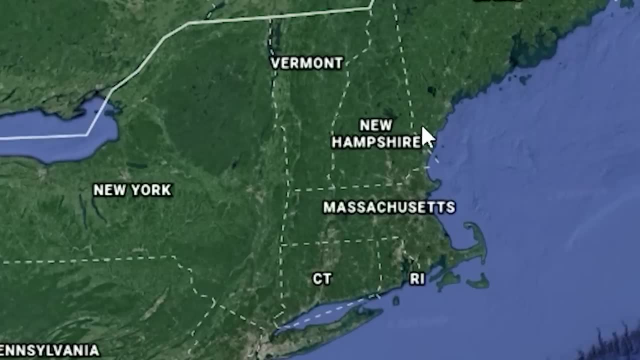 not a lot of population, It's it's flat. You know it's very easy to invade flat places and you're in the middle, You're not leaving like safety, you know, cornered off by the sea. That's tough. And then, short of New England forming New England, I don't think these states have much of a chance. 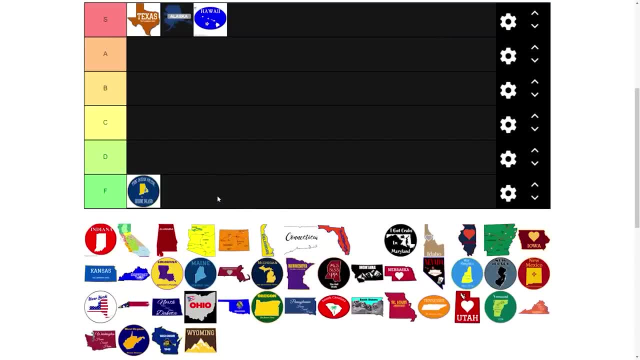 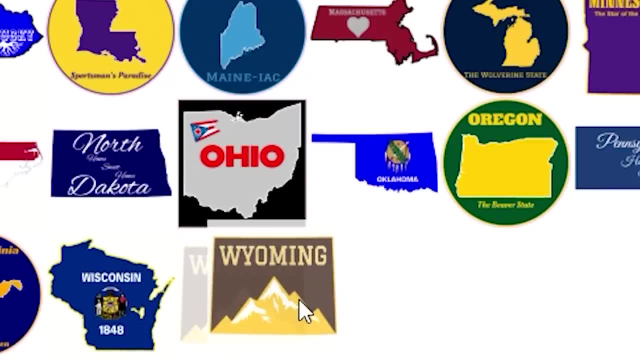 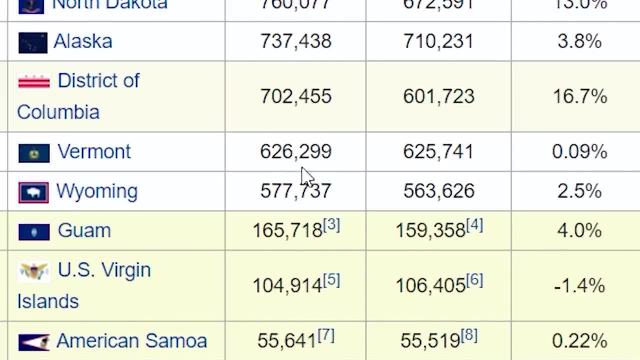 either- I'm sorry to do this to you- Rhode Island, But yeah it's tiny, And yeah, I'm sorry. Same for Wyoming, And it's just because you got no population And I just Yeah, it's just Sorry. guys Wyoming Vermont, I mean, Yeah, their situation Now at least Vermont has like a big 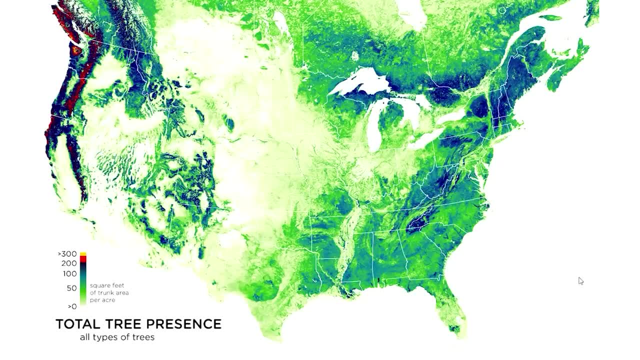 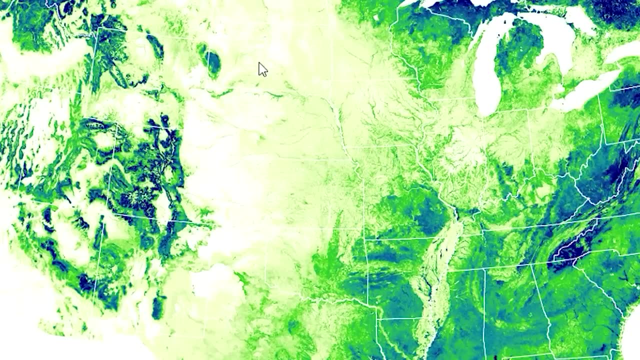 forest right Isn't very foresty- That that would help them. I got a little map here talking about trees and things like that. So I do think, like I said, at least New England and the east coast has all this. Again the middle of the country. Not fun. Hate to do this to my birth state, But 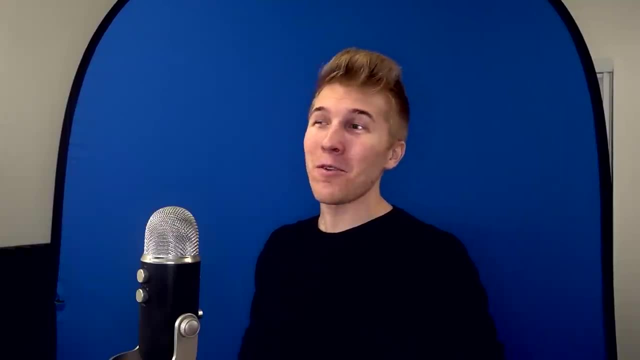 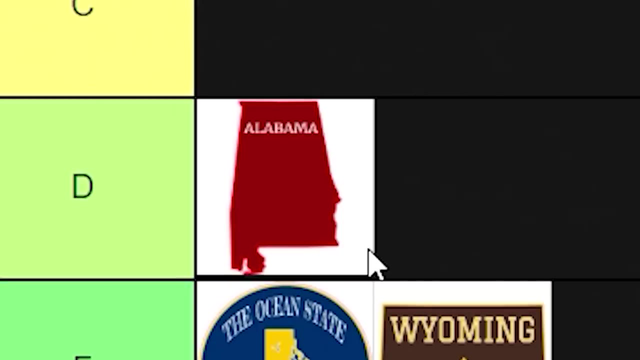 you know they're right next to Florida. I mean, if they were located anywhere else, I think they're just in a bad spot I'm going to. It's my birth state. I don't want to do this, But I guess I have to. I hate to do this to some of you, But being so close to Texas, New Mexico, 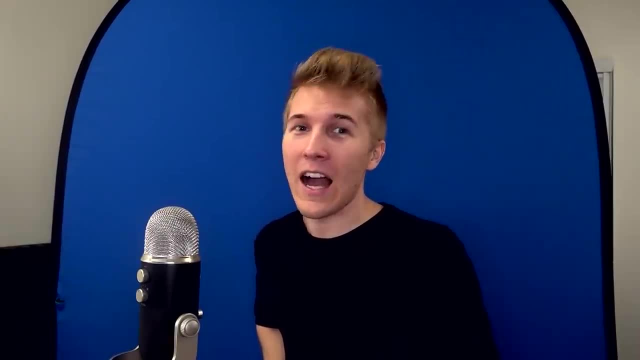 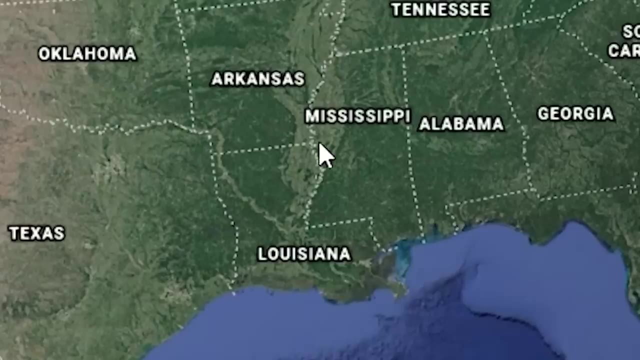 Oklahoma. Oh, it's going to make a mad, Like you guys hate Texas a lot Like people around Texas, But you're right next to him. I just can't see you surviving for that long. Maybe Louisiana- I do have you know like Louisiana- might be OK. They might be able to hold strong for a little bit. 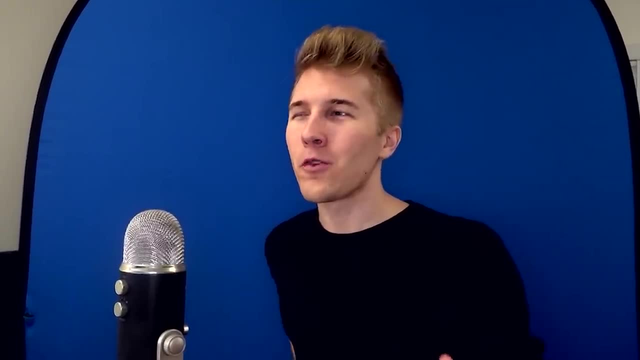 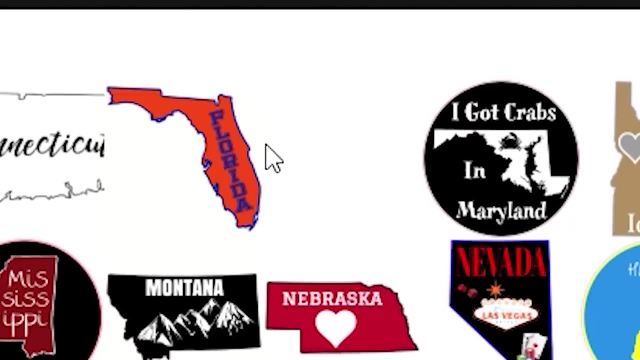 Again, this is like a free for all, Like obviously, you know, in a real Life scenario there'd probably be like alliances that would happen. I'm just going to assume it's just everyone for themselves. I feel like Florida obviously would do really good, especially from the. 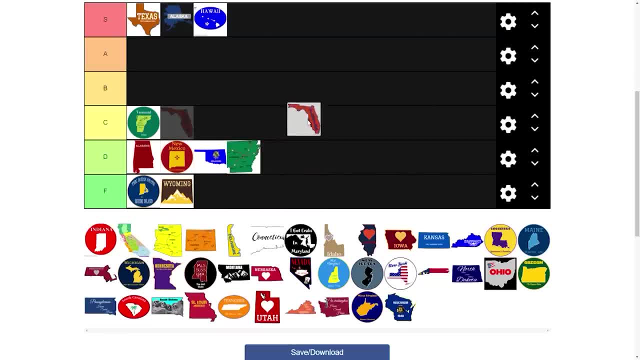 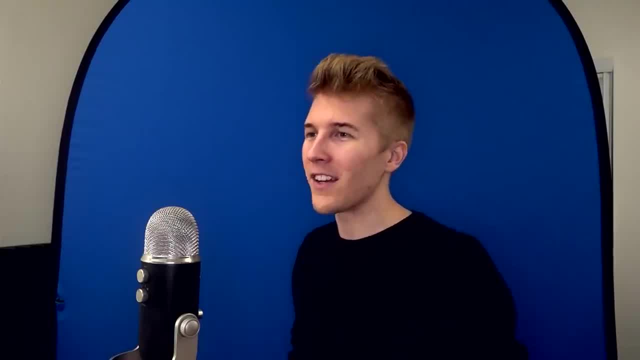 corner there until they meet Texas or someone- North Carolina, Virginia. I think would give them some tough one A B or an A Somewhere here Who went between New York and Pennsylvania. Yeah, I feel like Pennsylvania would have to worry about some of these neighbors. New York would be. 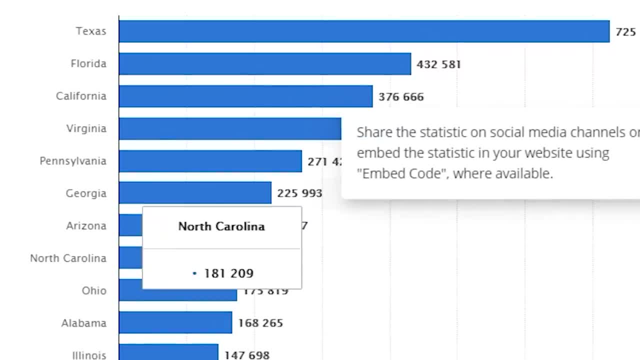 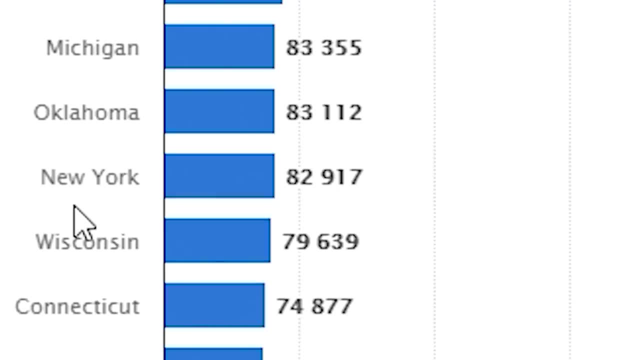 a little bit better. I don't know. Oh, maybe Pennsylvania wins Right there. Where's New York at in terms of This thing? Oh dang, They're way down there. Oh man, OK, Maybe that's the factor we got to think about. 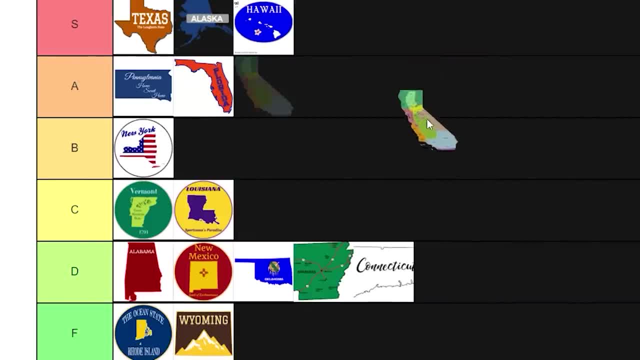 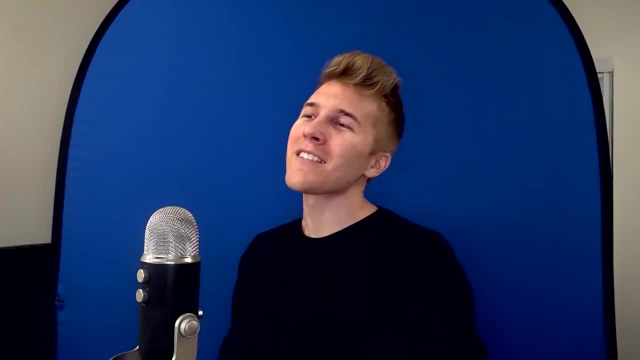 Oh man, let's do it. This is a hard one. California, Where is my state going to go? I mean, they're not going in A or S, I just can't. They're just. The only thing they got is a lot of population, I'm assuming military bases. 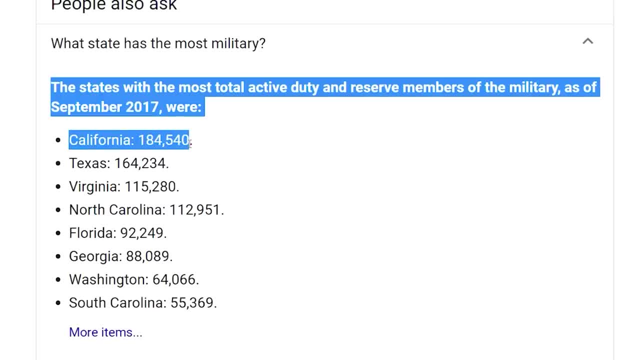 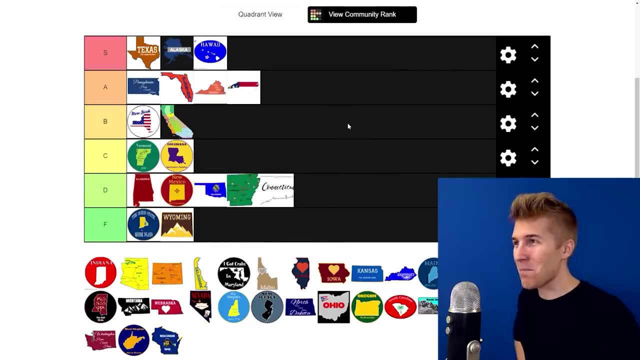 I don't know if we should count those. I did look those up. Here's like active duty, But Oh See, yeah, These two high up there too, I don't know. I feel like purely just based on people alone, I'll put them in B. 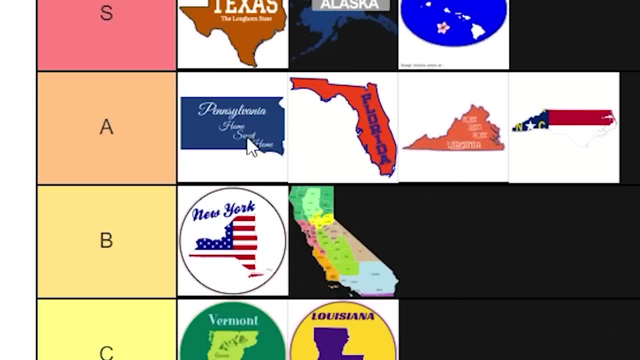 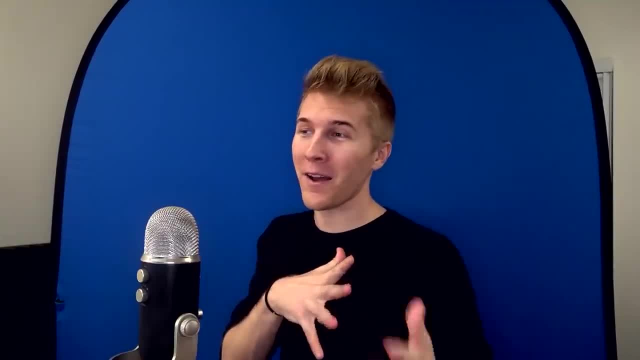 I think these states definitely would do better. I don't know. I'm kind of just like going. I'm just throwing things out there, So who Tell me? Don't forget to tell me how wrong I am, because that's definitely gonna be a thing. This is random, but I feel like West Virginia would do better than we're. 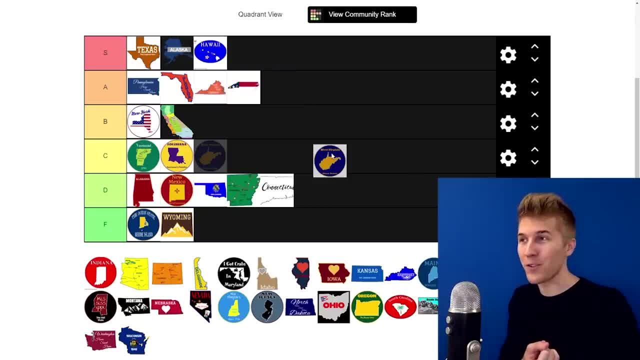 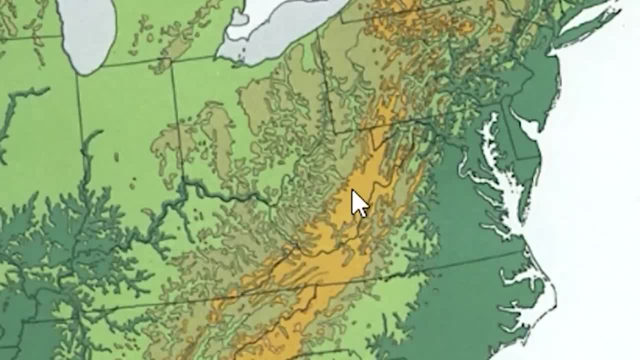 all expecting, You know, because they got the, They got the roads And obviously the mountains, But mainly the mountains. I think the mountains would help Like boom. they can just turtle, like the Swiss, Like Switzerland, And they might be OK. I mean, Virginia would probably, I don't know- North Carolina too. 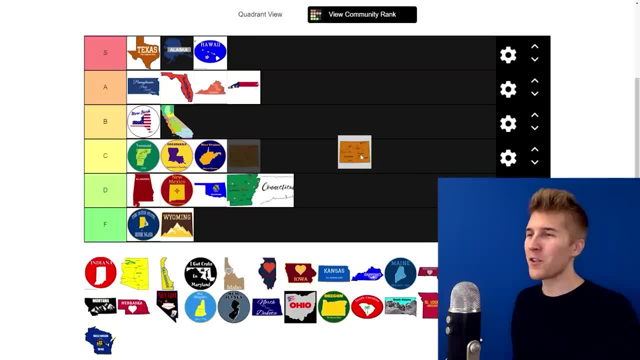 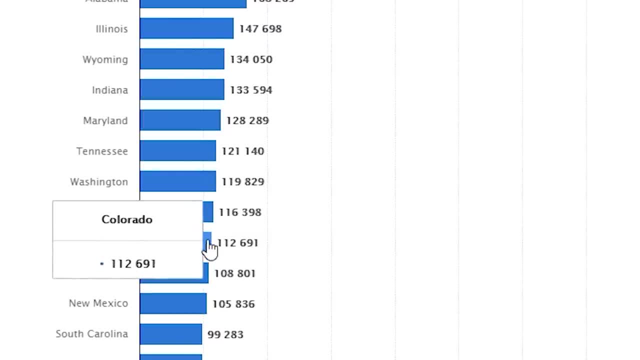 That's why these states would do OK. I think Colorado would maybe be an underdog as well. Hold on, Let me look at some things. Colorado don't got a lot of people, And they actually are a little bit lower on this list than I thought, But they got the Rocky Mountains. That helps. 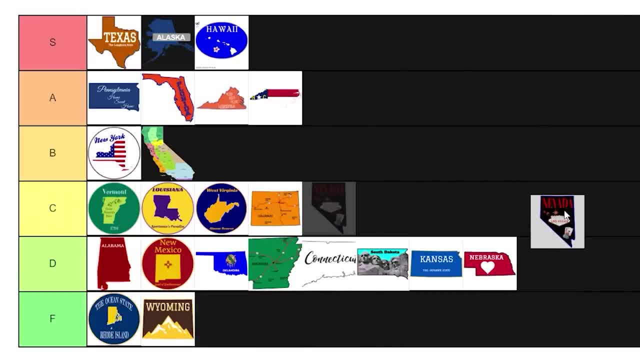 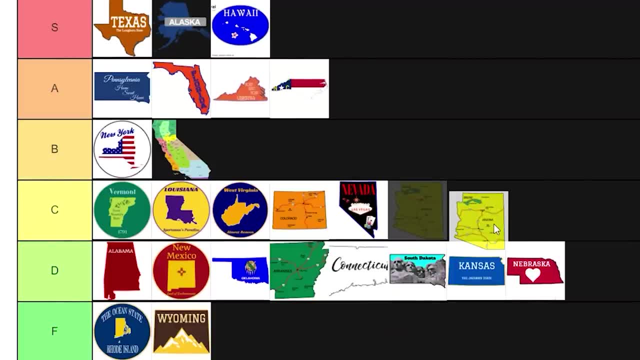 I feel like Vegas would be able to seduce enough people with some illegal narcotics and maybe some floosies. I think Arizona would be good too, But being next to California, I think they would hold their own. Cascadia would not be fun at all to go after. Look at this. I mean Oregon and Washington. This is why I think California, Maybe California should go even lower. if not, Because, like all these enemies next to them, That would not be fun. Nevada, I think they could get, But you don't want to go up into into here Like that's, that's gonna be bad. This is where things are gonna get tough Because we got like Michigan, Georgia, Ohio, Illinois. You know they got a bunch of manufacturing over there So they'd be pumping out those weapons. Sorry, South Carolina, But being in between Florida and North Carolina That'd be tough. Maine and Vermont are actually really low. 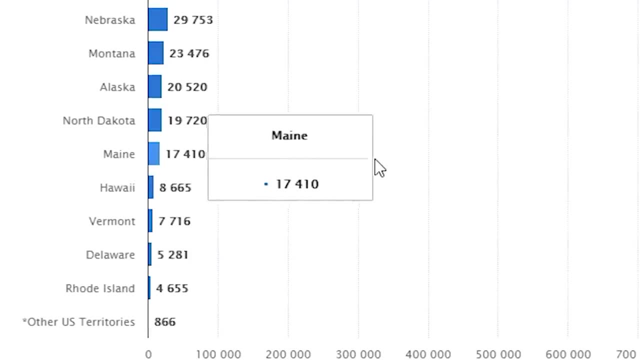 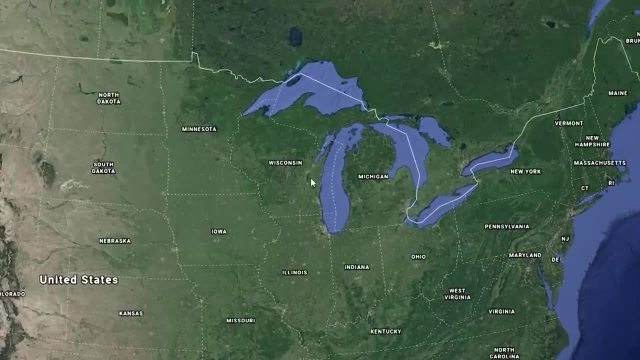 on this arms list, And Delaware And Rhode Island. Oh wow, that's not good. Yeah, this is like the toughest region to call. Like who comes out on top in this region? It's two like Illinois, Indiana, Ohio, Michigan, Wisconsin. 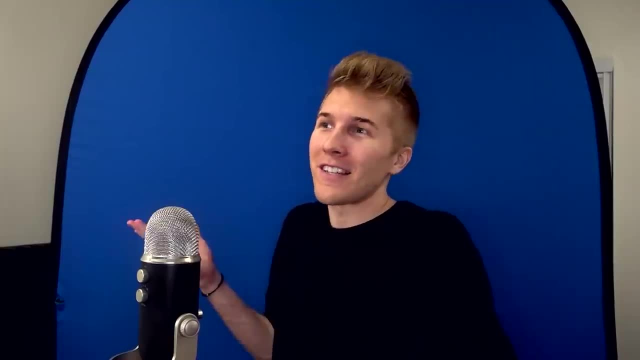 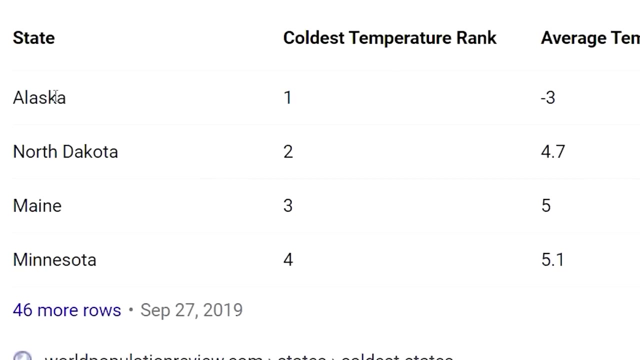 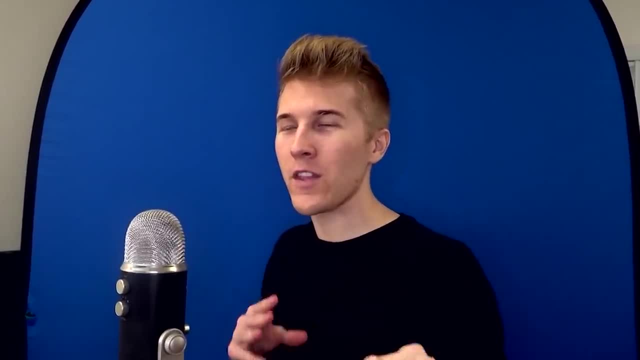 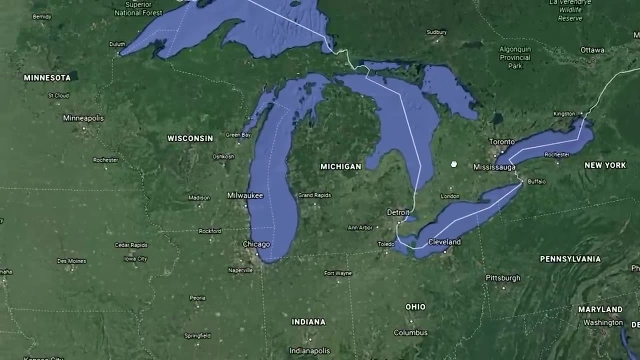 Maybe, Because maybe if they set the chickens free and then they train the chickens, Maybe put like a little- uh, explosive device- I want to say purely because Michigan is cornered off- they might be in the best situation, Although they gotta protect two different areas and that wouldn't be fun. 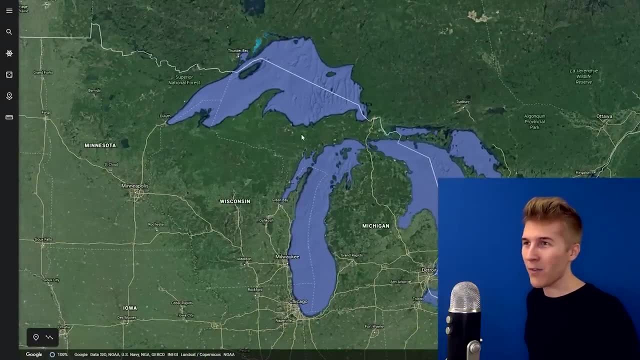 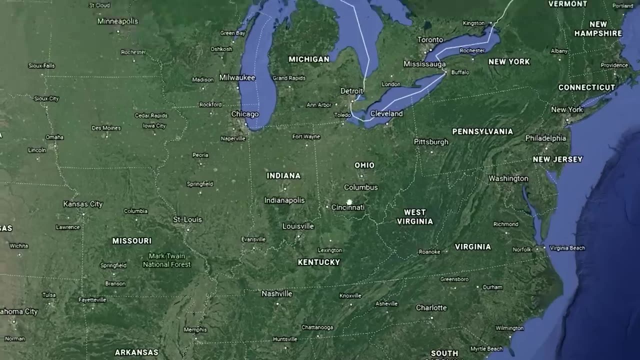 Maybe you just let you know Wisconsin invade and you just try to hold them off. it's gonna be cold up here too, though you gotta stop hope Indiana and Indiana Ohio got a deal with Kentucky and air all their surrounding neighbors. yeah, I think Michigan would be pretty good, but Minnesota to Minnesota may be. 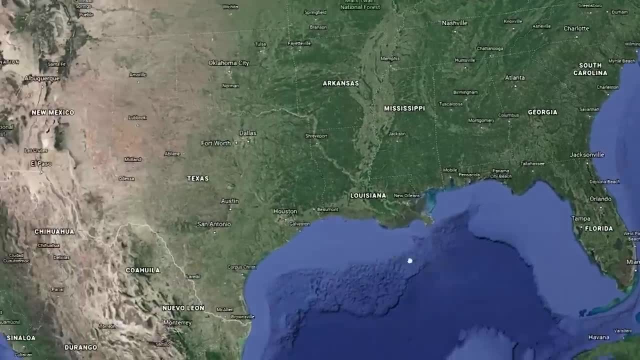 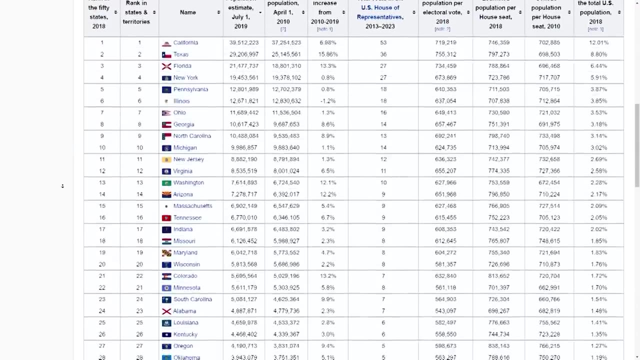 maybe I don't know. this is really hard. this is actually really hard because it gets like super, like in the middle. you just you can never tell what's gonna go down. I probably would have ranked most of the Deep South a little bit higher, but yeah, like I said, because of their situation, all smashed between a bunch of 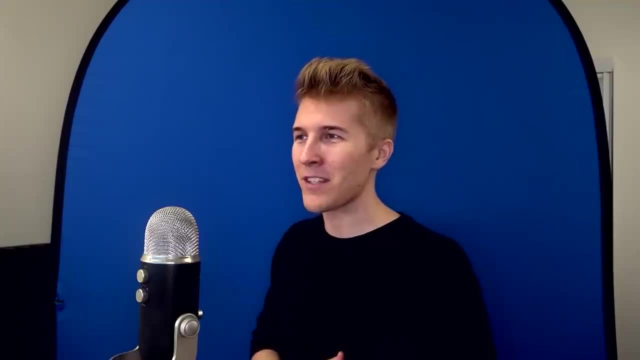 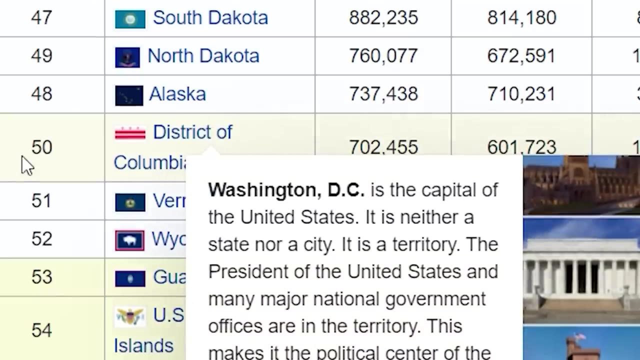 other really probably good states. I think it maybe brings him down. oh, should I? Puerto Rico's not on this list now. I don't think Puerto Rico would do well DC. DC has no chance. well, they have less than a million people, so that wouldn't be fun. Oh, Alaska does too. I didn't realize that. but again, I mean, you don't, you don't. 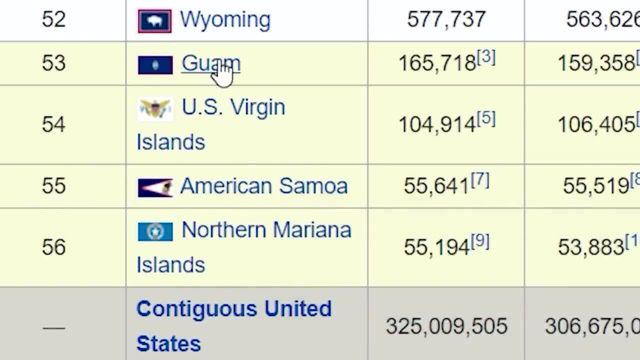 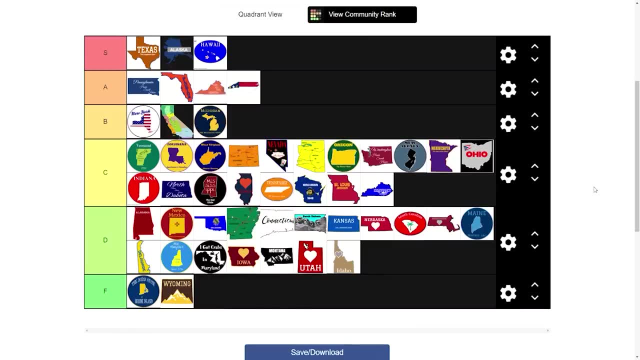 want to go there. America, Samoa would be super safe, and so would a lot of these, yeah, a lot of these dang America. so, oh, it's 55,000 people right now. I definitely am NOT a hundred percent sure about these ones in the middle. I want to. 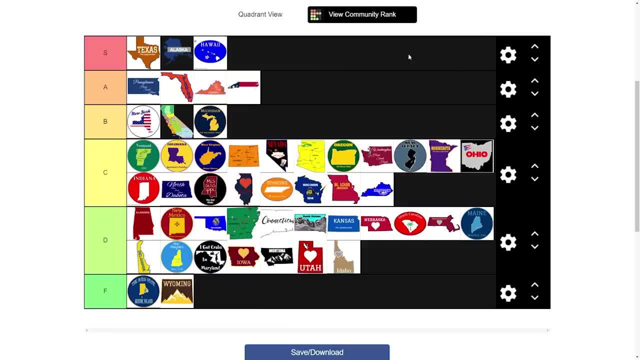 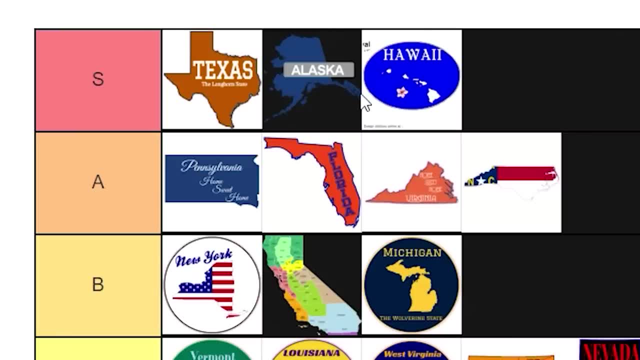 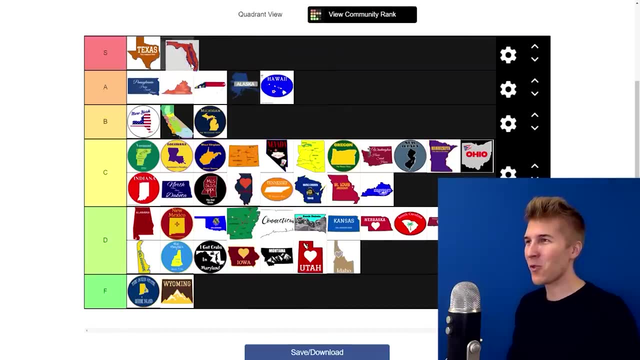 make a lot of adjustments, but I feel pretty strongly about the other top part of the tier and the bottom part of the T. actually it's really weird because having Alaska and Hawaii so high- but I think it's by default, right, it's kind of by default. it really should probably be this. maybe Florida up there, maybe. 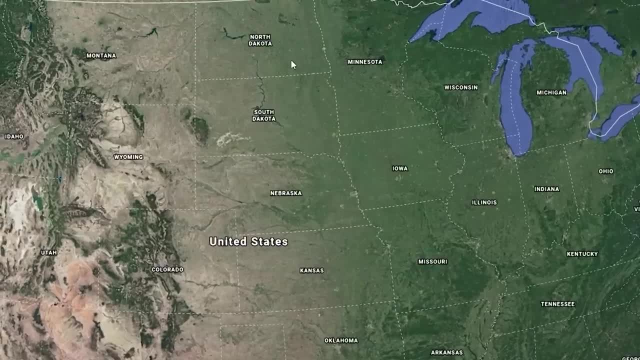 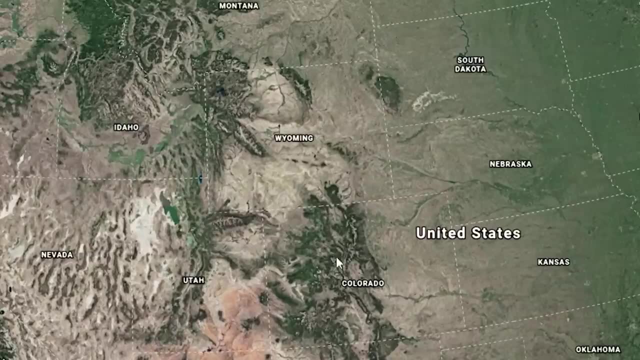 Virginia, North Carolina. like I said, this part of the states it's gonna be tough, although as you get higher up here, the cold is gonna affect them. these days are okay, but they don't have a lot of population. that'd be the biggest problem here, but they at least got the mountains to protect them. Oregon and Washington: I. 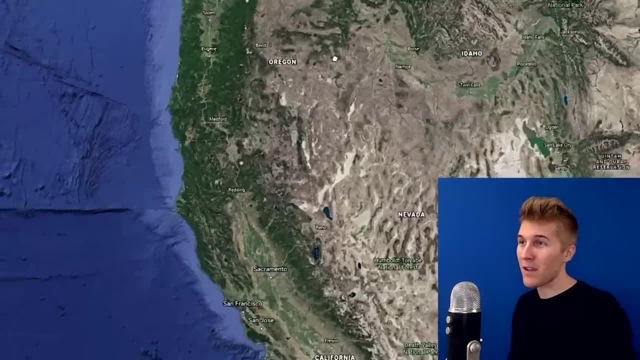 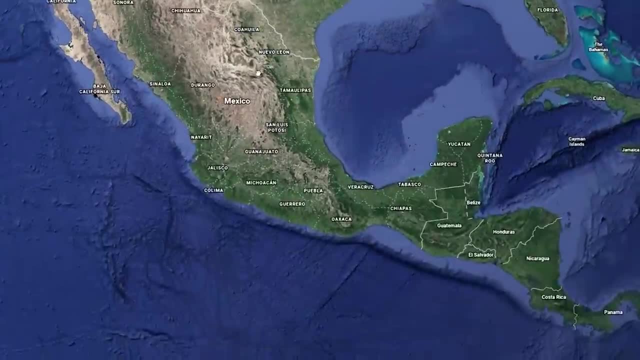 don't want to underestimate them, because Cascadia would not be fun. that would be crazy, like it'd be California's Vietnam. everyone near Texas would be kind of in trouble, especially cuz Texas is walled off. Mexico is not gonna get involved in this scenario. they'd be able to spread out. I think Louisiana would hold strong. 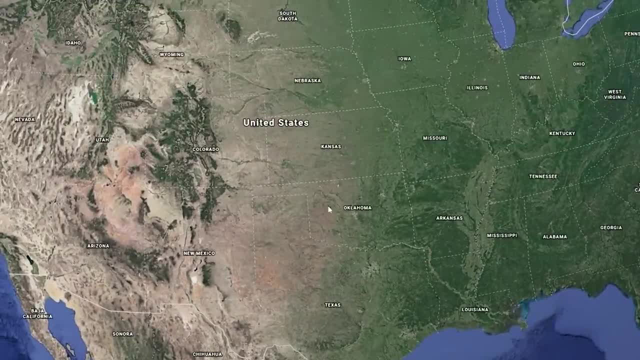 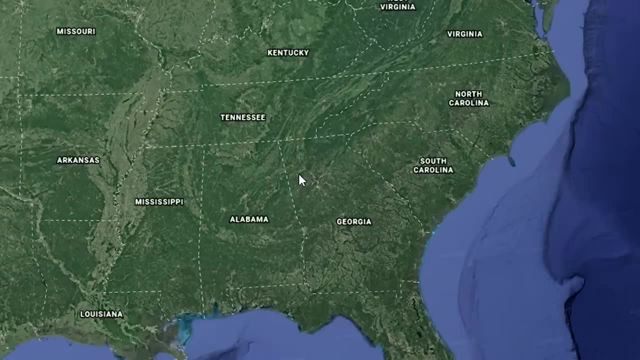 for a little bit, but Texas would definitely take a lot of this. maybe if they, if Texas, moved toward the west coast, they'd be really good. this would be too much of a cluster. I think it's too much of a cluster to know at any point. anyone could come out on top here, though I really think anyone Florida. 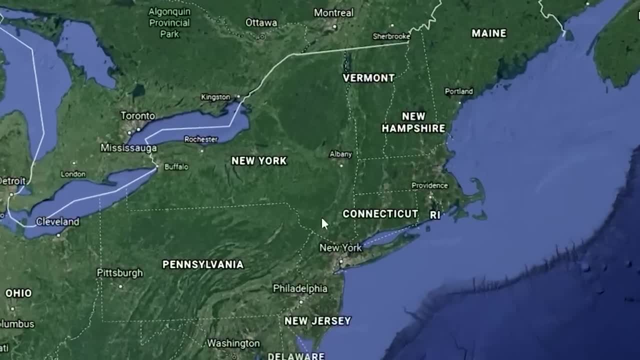 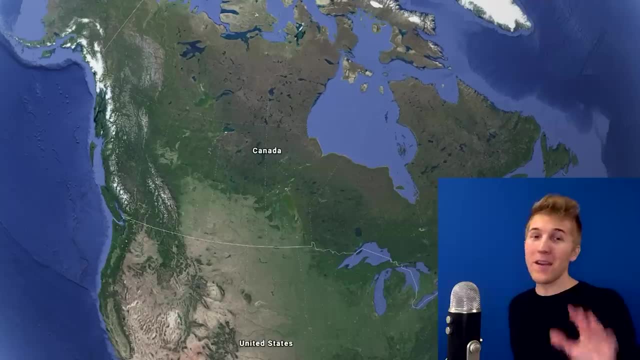 would be tough. and Georgia to actually New England, yeah, I don't know. I mean, unless New York's really distracted by the cold, it's gonna be a lot of trouble. but Pennsylvania, this is hard. but they can manufacture a lot, that's, that'd be my kind of guess. this would be a completely different scenario if Canada. 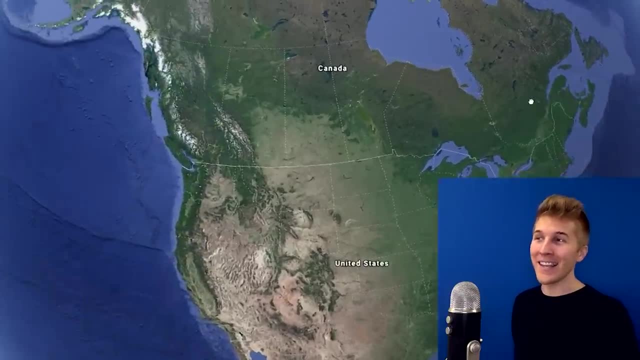 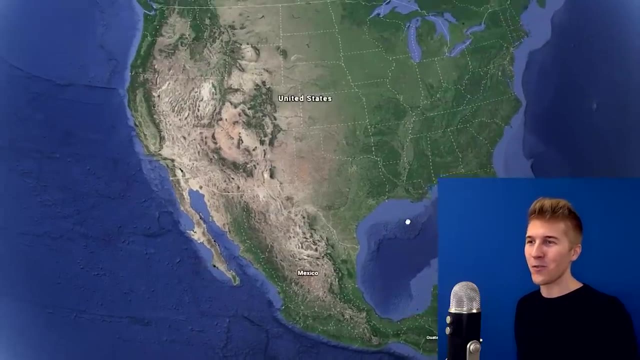 was up for grabs, though I think if Canada was up for grabs, then things change a lot. or if Mexico, obviously, if Mexico was realistically like involved too, which I mean it's a battle royale, why wouldn't they? and then the Europeans would just be chilling. there'd be, finally, the ones that would be like you. 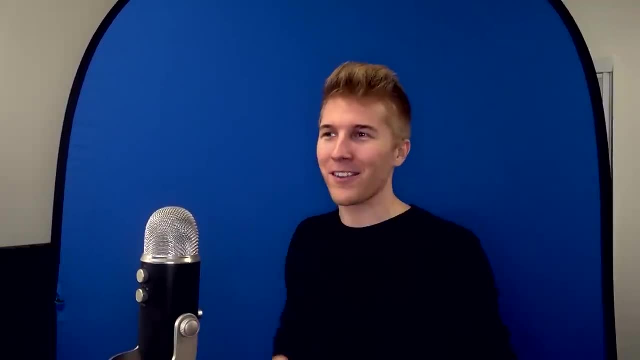 know, just kind of watching, observing, seeing what's going on, Oh, like with binoculars. oh, I don't know, I want to make some adjustments. this is not my. I want to think about this. I'm gonna think about this for a long time, but yeah, I. 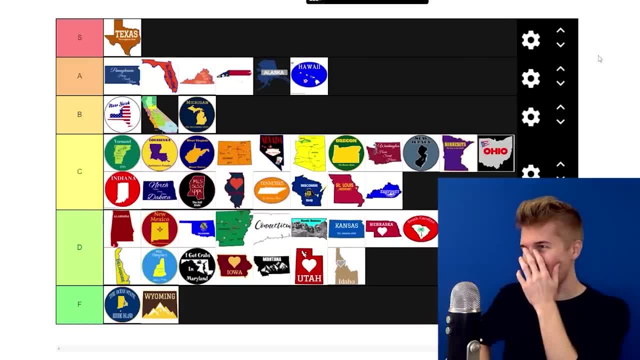 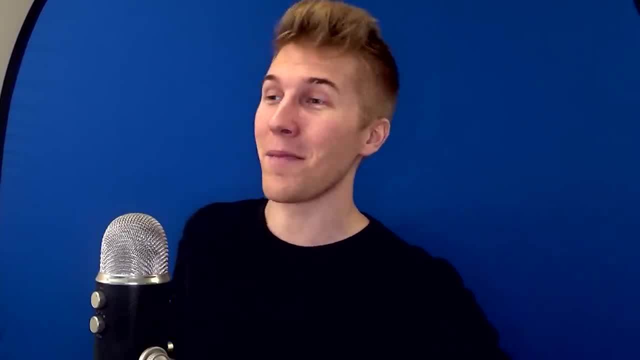 can't. I got it. I got to move on. I'm gonna regret this, but yeah, sorry if it put your state low, let me know down in the comment section why I'm maybe wrong. there's probably some other fact. there's actually a lot of factors. I'm not. considering, but I didn't want to use like military bases because like would those bases technically, I guess they would fight for their own state, maybe not? it's too confusing. anyways, let me know down below. thanks for watching, see you next time and big thanks the January patrons: LVC, Elijah Senpai, Lucio for a vacation. Thanks again. 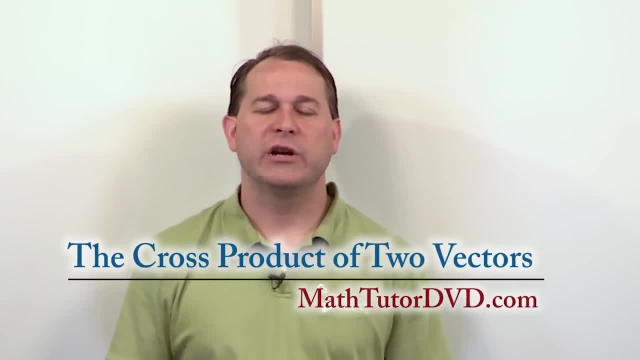 Hello, Welcome to this lesson in engineering mechanics. Here we're going to cover the cross product, and we're going to talk about the cross product in terms of math, in terms of the mathematical definition. We're not going to talk about moments in specific here, but I'm kind of giving you a little bit of a preview.